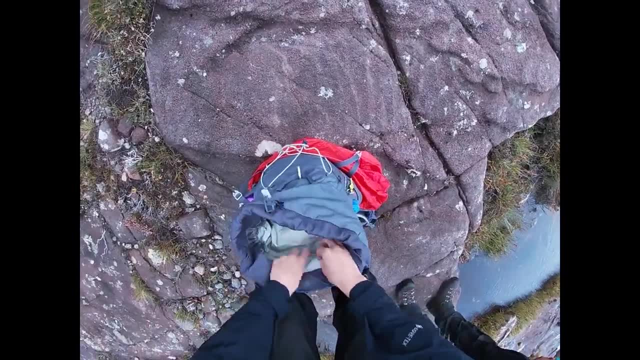 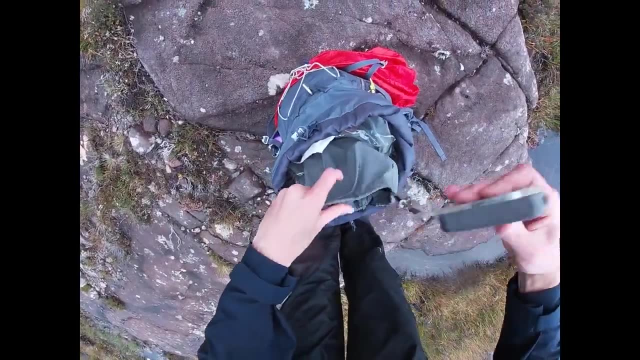 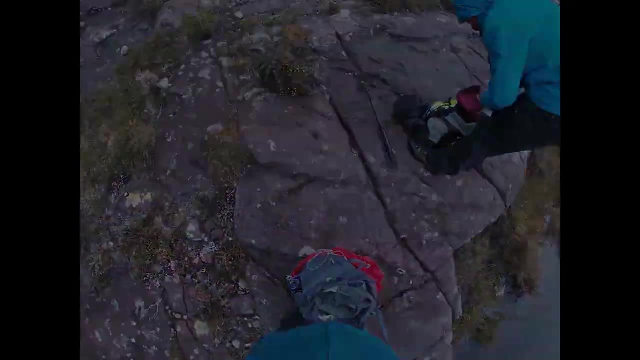 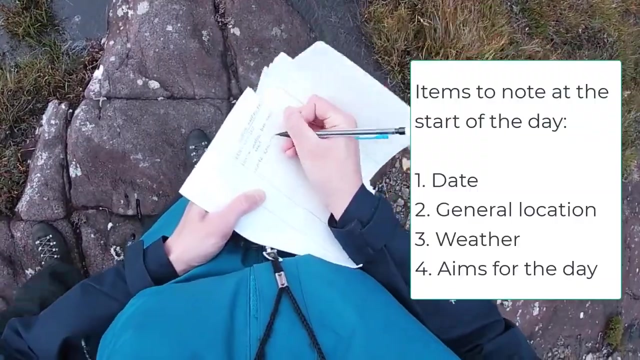 Now let's map This geological unit onto our geological map. So the first step is we need to get all of our kit ready. So we need our field notebook, we need our compass, we need our pencils, and now we're ready to document some of our observations. We start by noting down all the key items for the start. 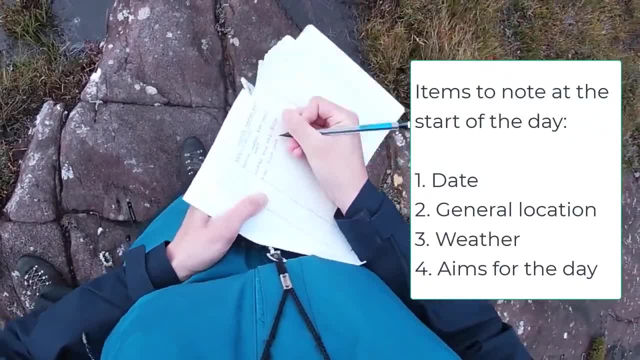 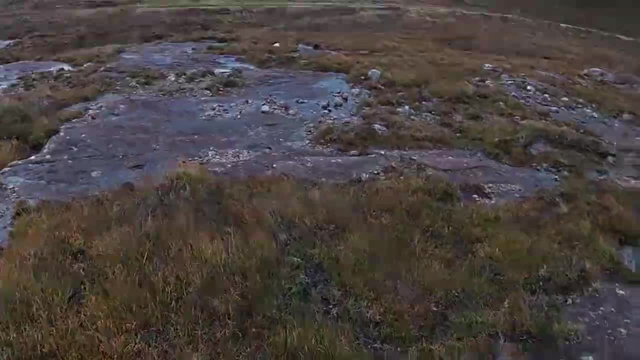 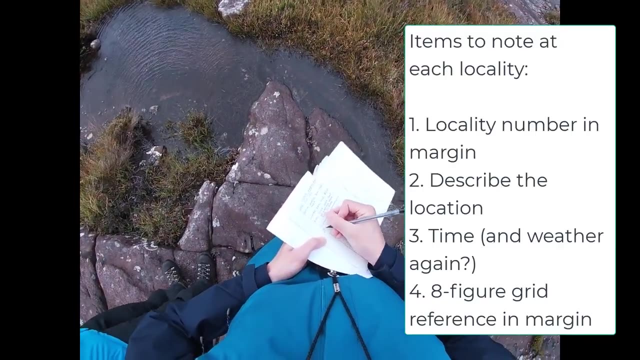 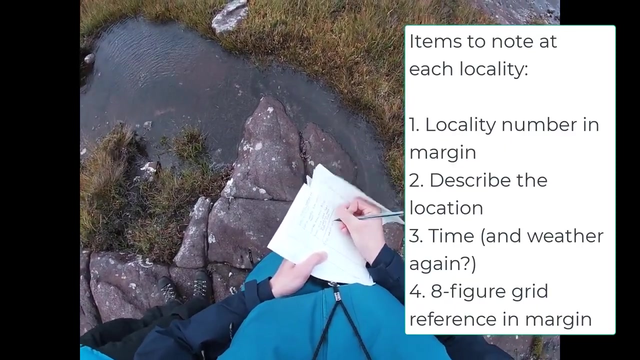 of the day, including the date, the weather, the general location, the aims of the day, so mapping out some boundaries in this case. Now let's start this locality. We start by describing where we are, so thinking about the fact that we're on these large flat slabs of brownish rock. So we want a brief location. 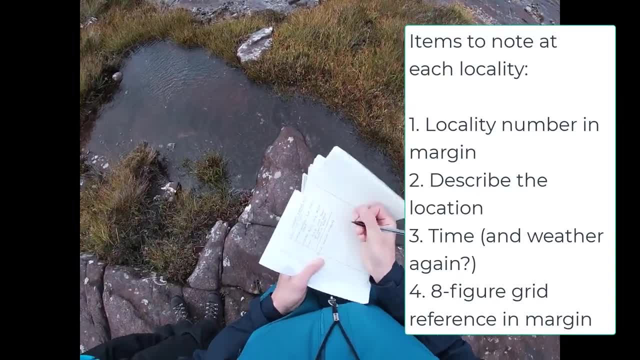 description for each locality and, of course, we will have a locality number that goes in the margin. Okay, so I'm going to break this down into the first part of the day. So I'm going to start with the start of the day and then I'm going to mark out the areas, or the women's areas, that we're going to get the information about. 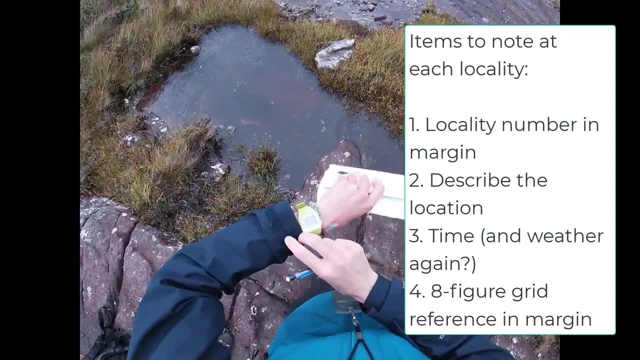 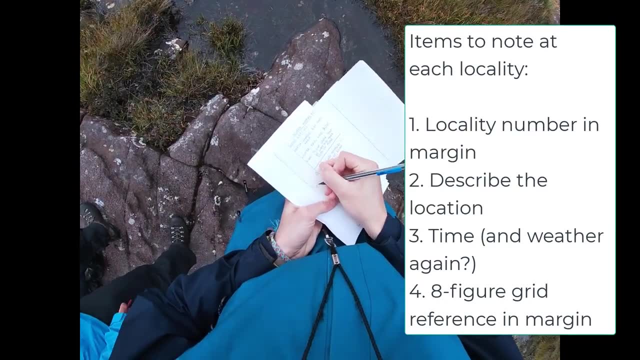 In this case, I'm going to start with the start of the day, so mapping out some boundaries. in this case, It is currently 10.17am. I'm going to write that in the margin. I've got my locality number 1.. 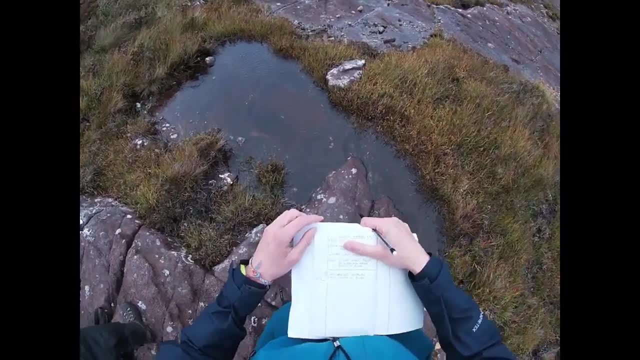 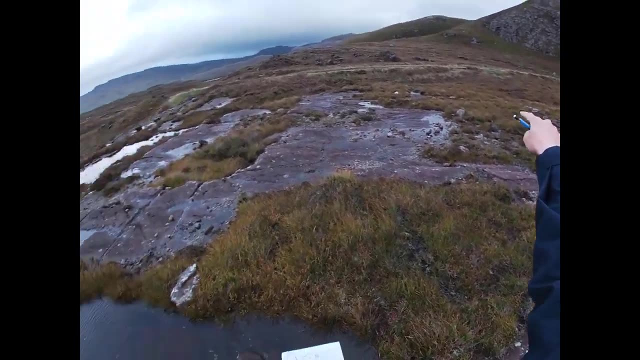 And what we need to do is now work out the grid reference. What we need to do to work that out is to think: what can we see around us? So I can see the bend of the road coming around, and there's another bend just right here. 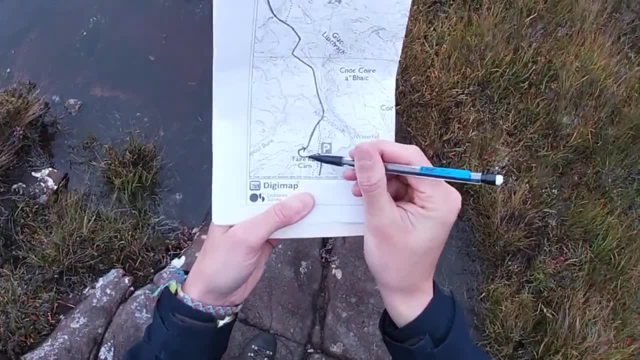 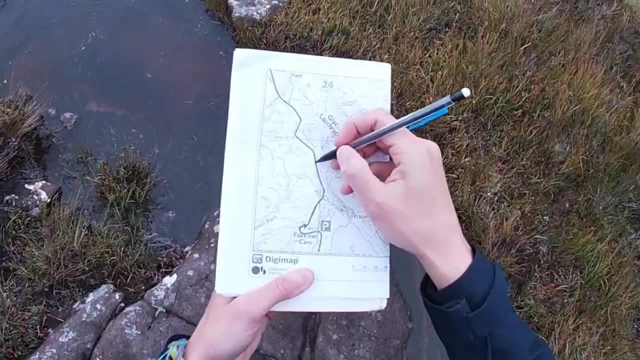 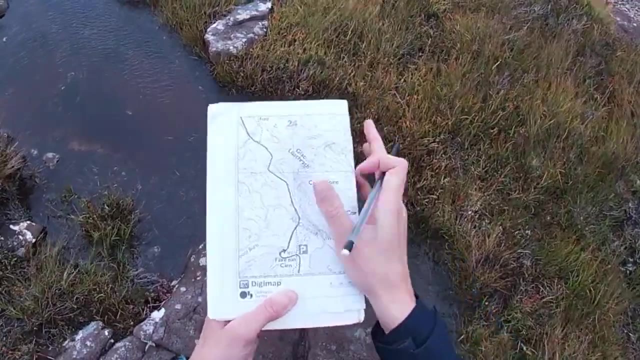 If I look on the map, you can see that there's that big bend which comes around. then we cross over a bridge, then we come down and then there is another bend and then a sort of sharp bend there. So the road- we've got the big bend up there- comes over the bridge. there's a slight bend and then a bigger bend. 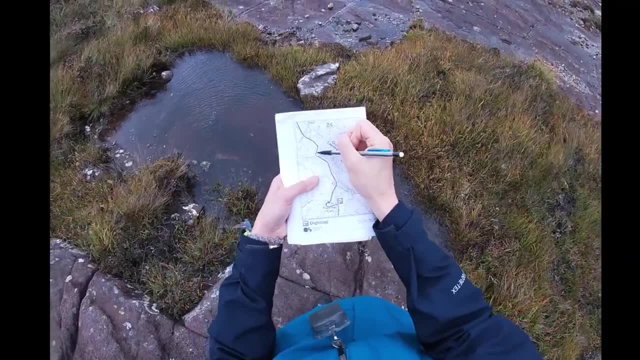 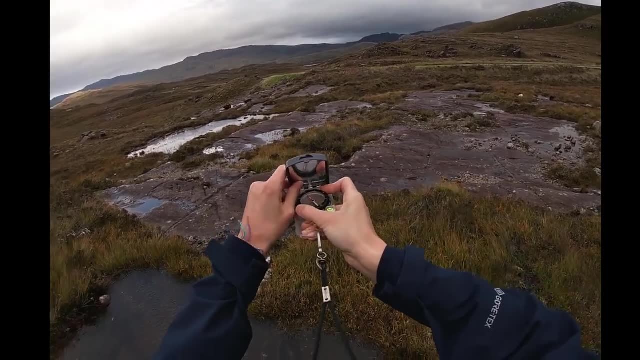 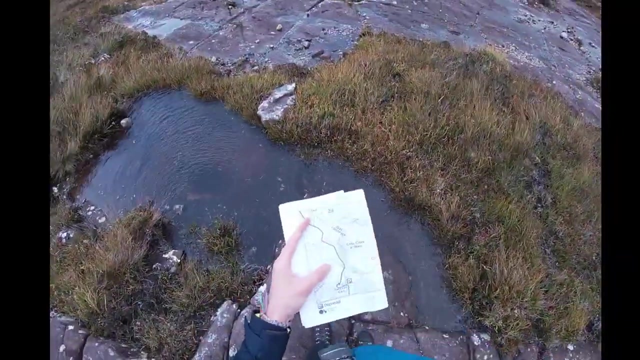 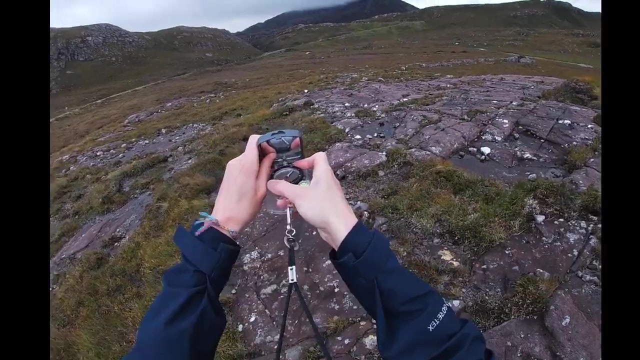 So I'm happy that I must be close to this bend To get a better idea of where I am. I will now take some bearings to those landmarks that I've identified on the map. So I'll use the sight on my compass, I'll line it up with the two bends on the map and then triangulate my position to be sure of my location on the map. 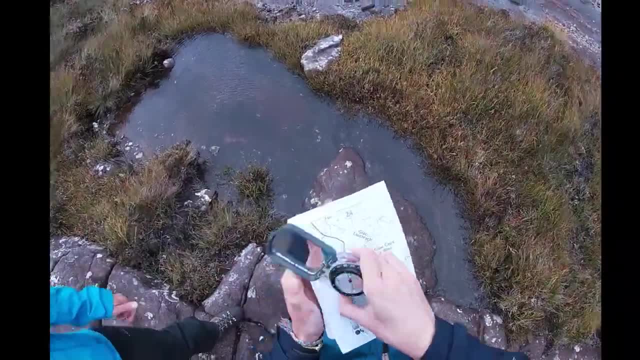 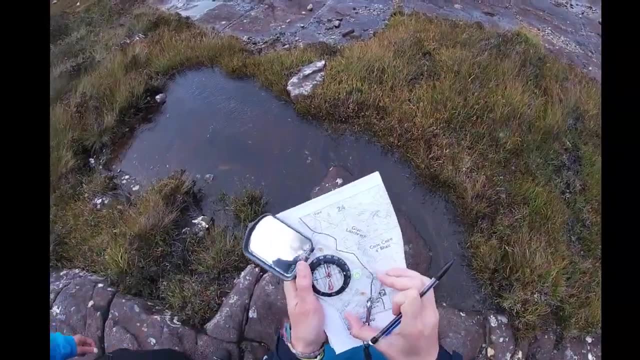 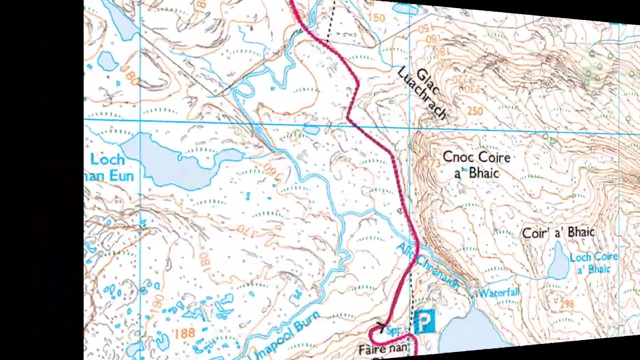 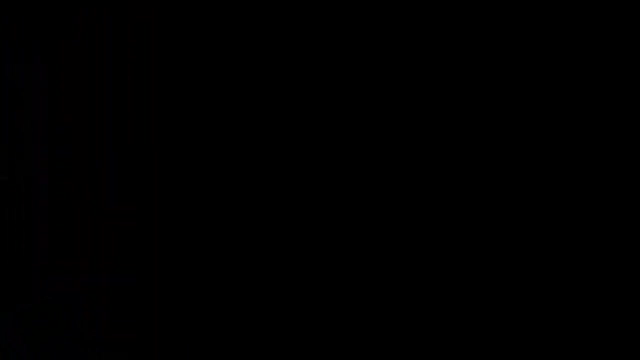 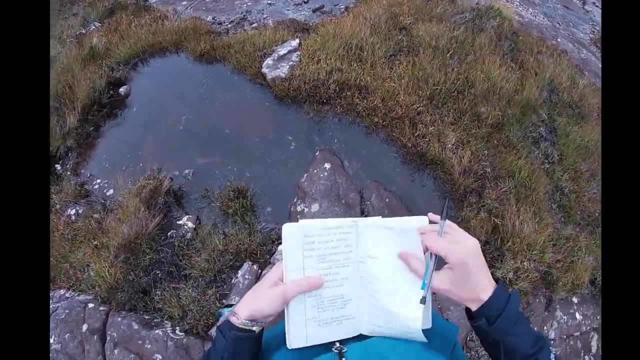 And by doing this triangulation we can sort of pinpoint where we are. It is then possible to work out a grid reference and write that down as an image. So I'll write that down as an eight-figure grid reference in the margin next to this locality. 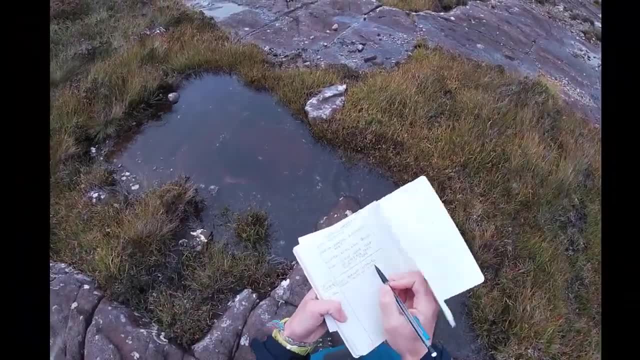 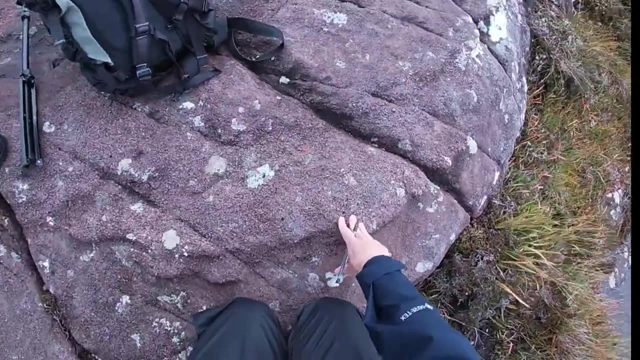 I've found where I am put my locality number, I've described my locality and I've put the time. Now it's time to describe the rock. I'm going to have a look at my rock- I might do a field sketch and I'm also going to describe it. 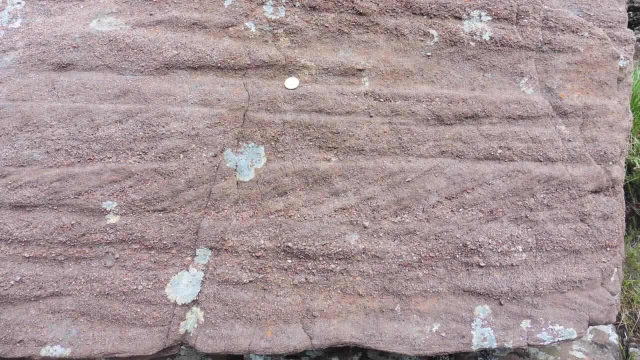 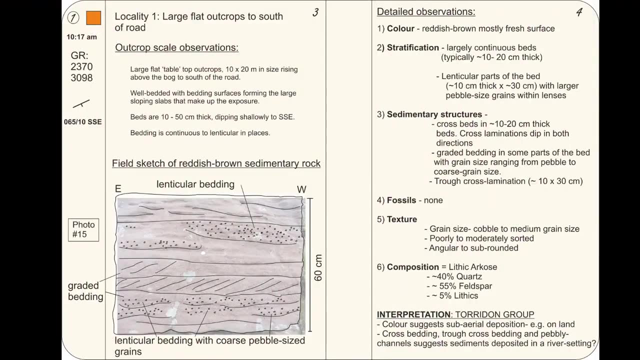 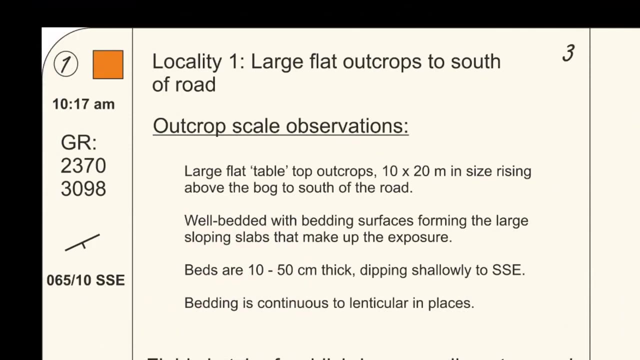 I make systematic observations of this rock type. So, looking at both the macro and micro scale features, I then systematically write these down, starting at the outcrop scale. So thinking about the fact we're looking at large sort of table size outcrops- 10 to 20 metres in size in some places. 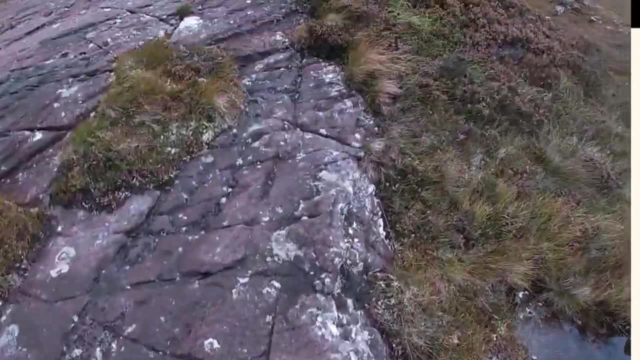 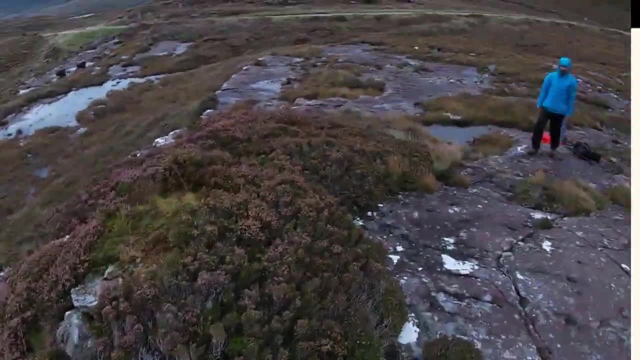 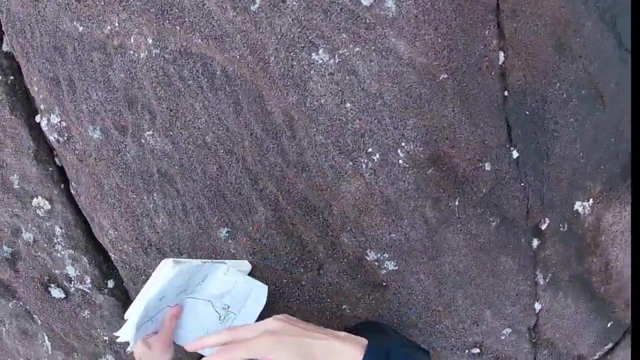 Obviously, some are a lot smaller, some are more on the order of a couple of metres. So we've got very well bedded sequence Of rocks where I am stood on these large flat outcrops. Now I'm going to take a strike and dip of the bedding surface. 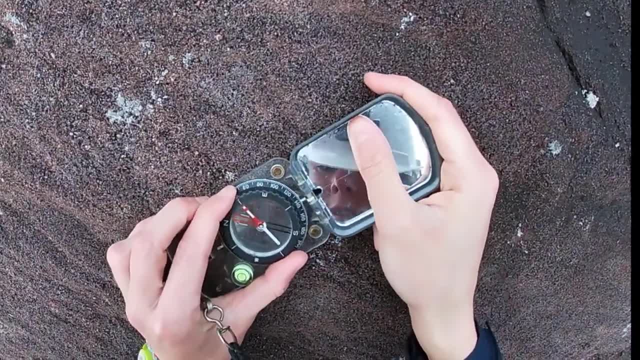 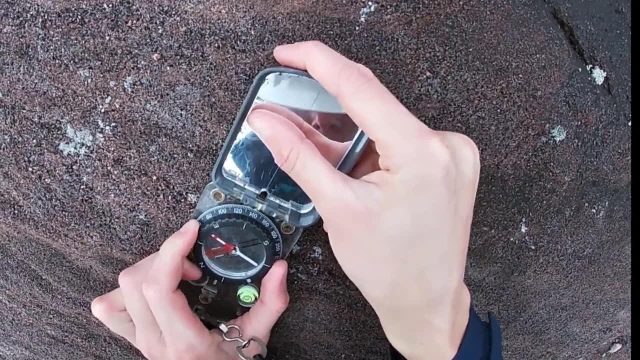 So there's some really nice planar surfaces here which are ideal for taking strike and dip. So I'm first of all finding the horizontal with my compass, So I'm using the spirit level on my compass to find horizontal. I am then going to rotate. 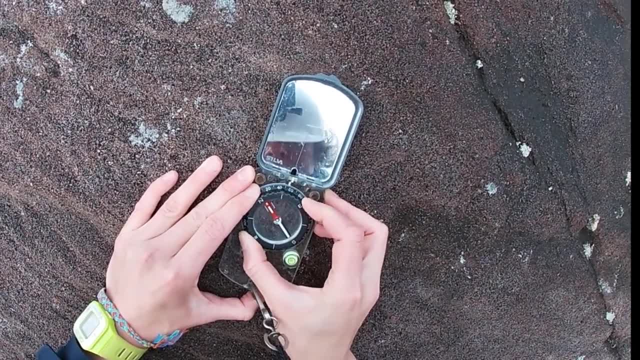 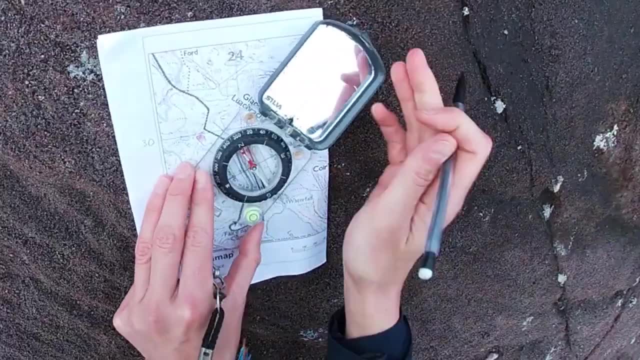 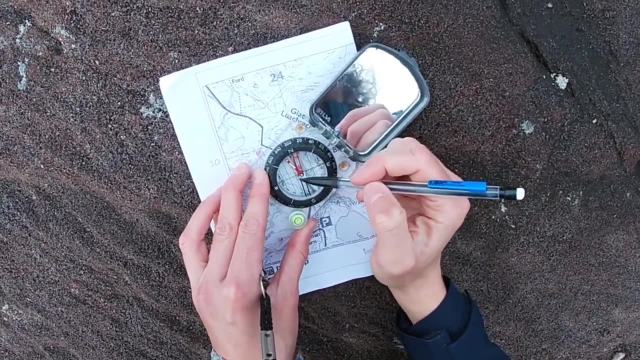 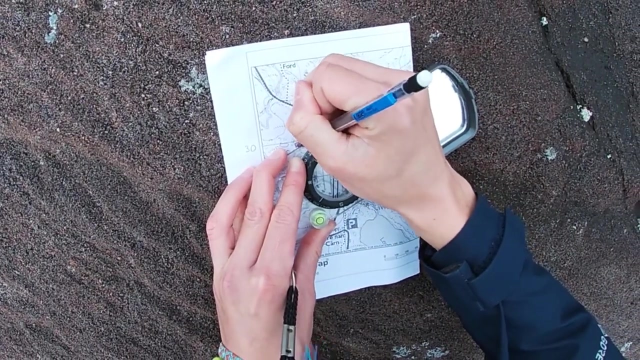 I indicate the compass housing so my north arrows line up. My strike is around 065 here Now with the torridon I would start lining up the lines on the bottom of my compass With the lines on the map. I'm just doing my little strike. 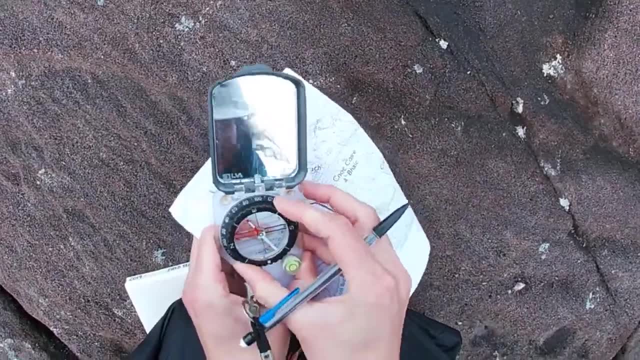 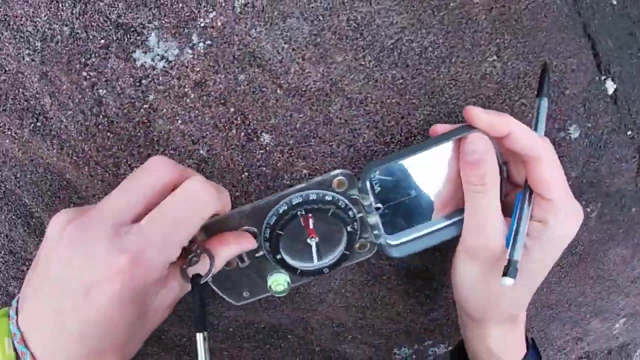 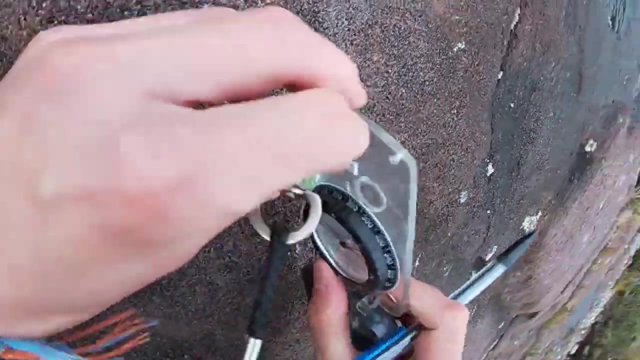 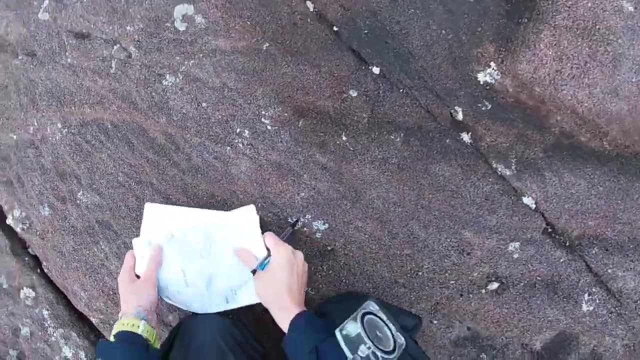 Now I need to work out which way it is dipping. So let's put that to 90 degrees. So if my strike was pretty much like that, I can even draw that on the rock foot, Which is dipping about 10 degrees. And we're dipping in this direction, which is towards the, basically to the south. 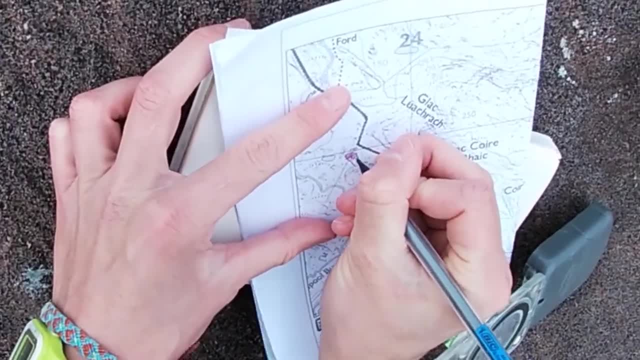 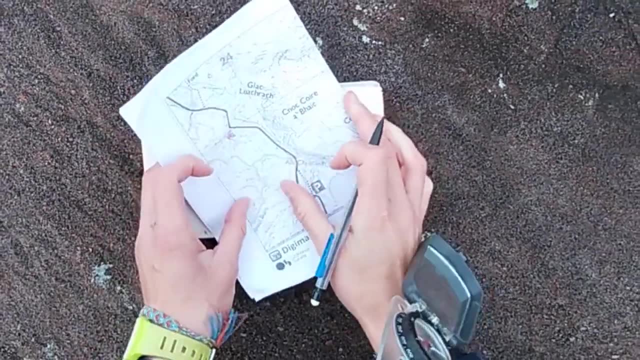 And I'm just going to write my 10 degrees next to that. So I've now got my outcrop, I've found where I was, I've drawn my outcrop And I've done my strike and dip symbol. I might put a little number 1 next to that. 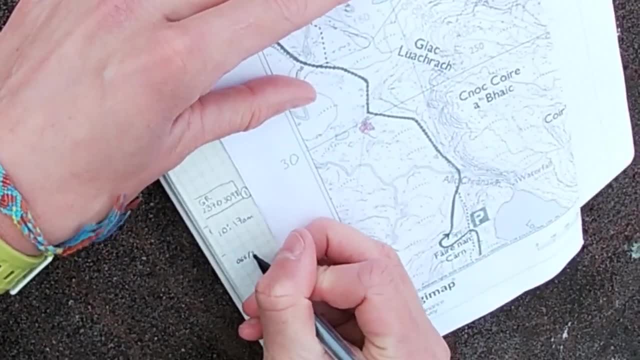 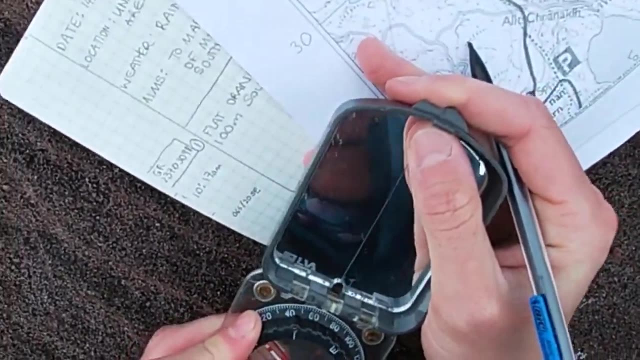 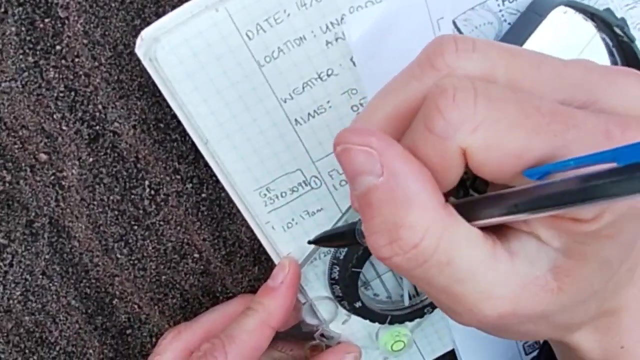 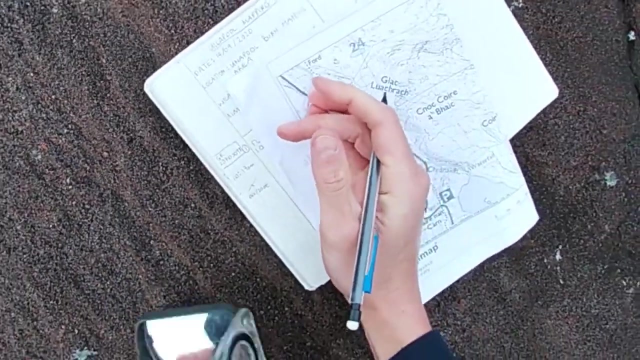 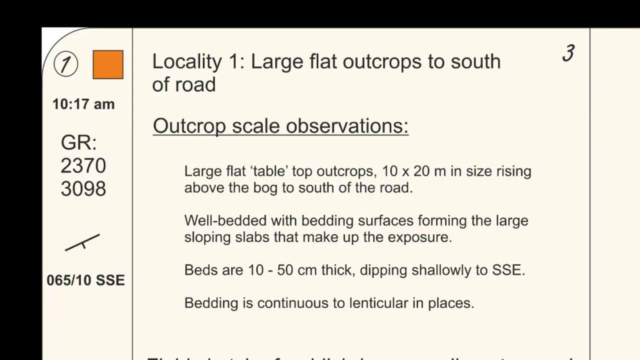 I did over here, So it was 065, 20 to the south east. And again I'm going to draw an oriented symbol. in here I've written down the thickness of the beds, The fact that they're shallowly dipping to the south, south east. 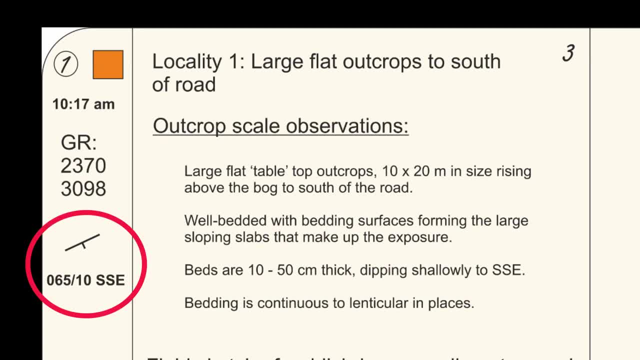 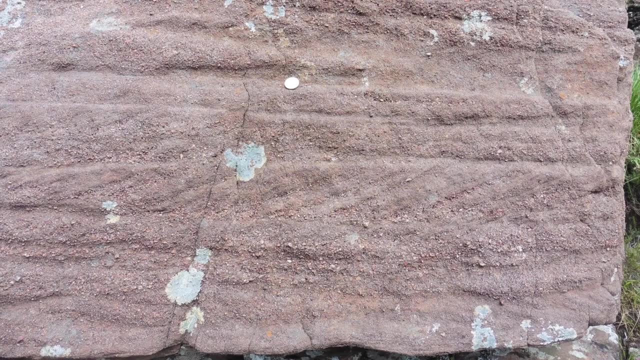 You can see the strike and dip symbol which is in the margin of my notebook. And thinking about the contacts with the beds, It's mostly continuous, Although there are sort of lenticular Parts of the bedding in places. You can now look at the features that we can see in the rock. 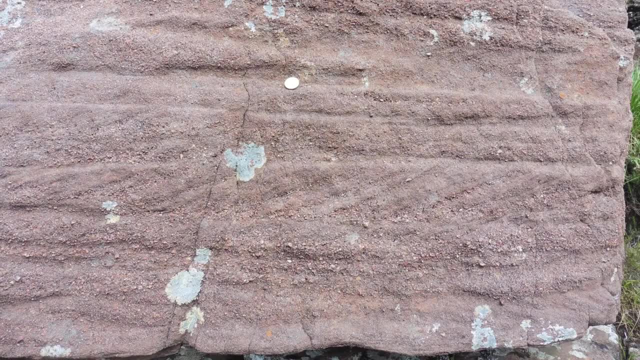 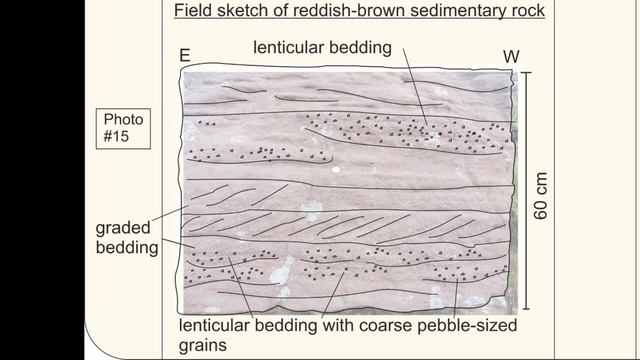 And I start off by making a geological field sketch. So I've noted some of the key features. So I've got a title on my sketch, I've got the orientation and a scale of 60 centimetres. I've then annotated some key points. 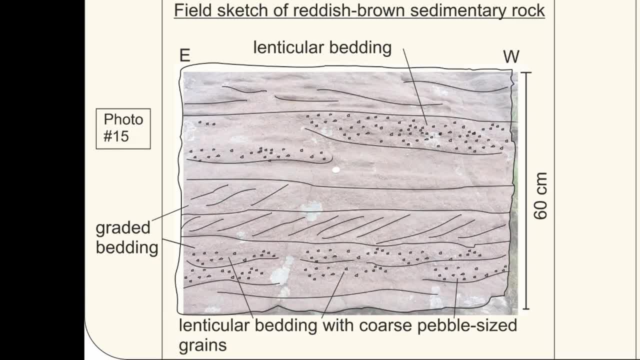 Such as some of the lenticular bedding, Which is the coarse grained part. So we've got more pebble and coarse grain size, Poorly sorted material. I've noted some graded bedding And some other parts towards the bottom of the outcrop. 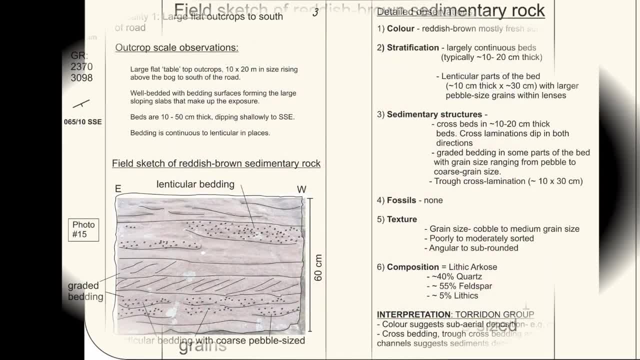 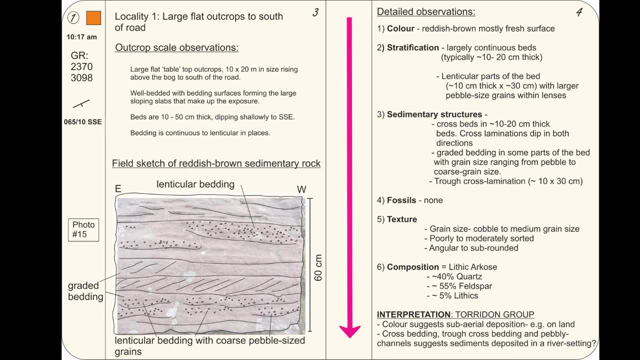 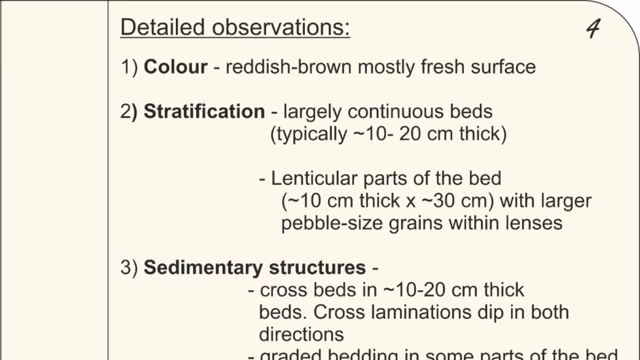 Where lenticular shaped contacts. Now we can do a detailed description of our observations. So I've systematically worked my way through a series of observations Which I've written down with subheadings. So, starting from the colour, We've got this reddish brown. 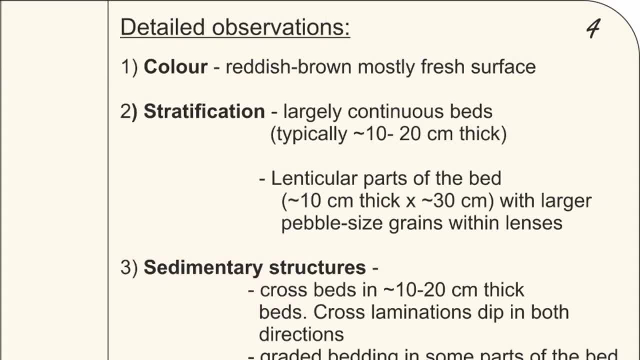 Mostly fresh surface that we can see on the rocks Stratification. We've got largely continuous bedding Which is about 10 to 20 centimetres thick, But it is lenticular in parts And these sort of lenses are on the order of 10 to 30 centimetres sized. 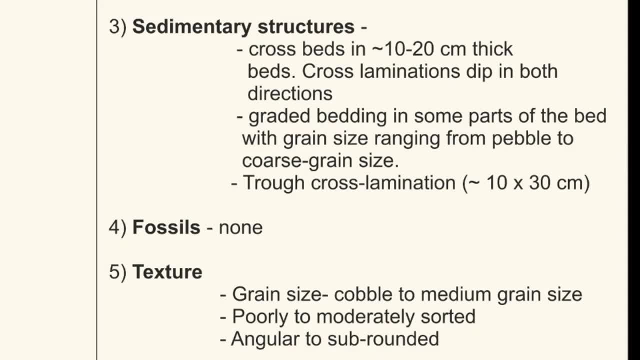 With larger pebble sized material. within those lenses, Sedimentary structures. I can see cross bedding in sort of 10 to 20 centimetre thick beds And laminations which are dipping in both directions In some places, Although in others we've sort of seen a uniform direction. 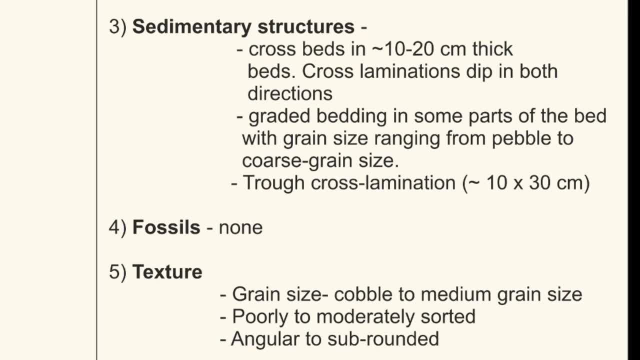 There's graded bedding in some parts of the bed With grain size ranging from pebble to coarse grain size. There's trough cross laminations as well. Can't see any fossils. The texture is the grain size is cobble to medium sized grain. 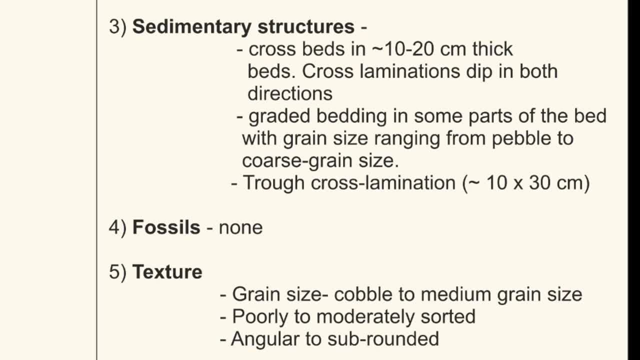 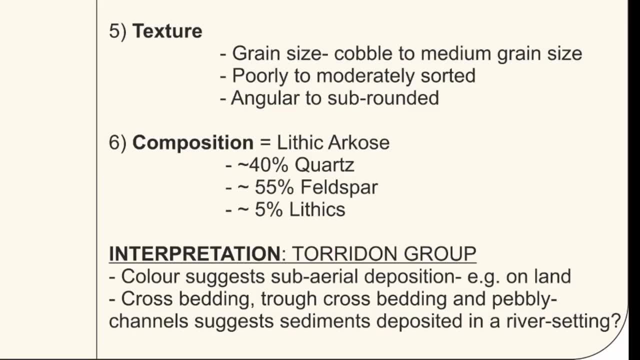 It's poorly to moderately sorted, Angular to sub-rounded. An average composition is about 40% quartz, About 50 to 60% feldspar And some lithic, So probably 5 to 10%. So this sort of classifies it as a lithic archos. 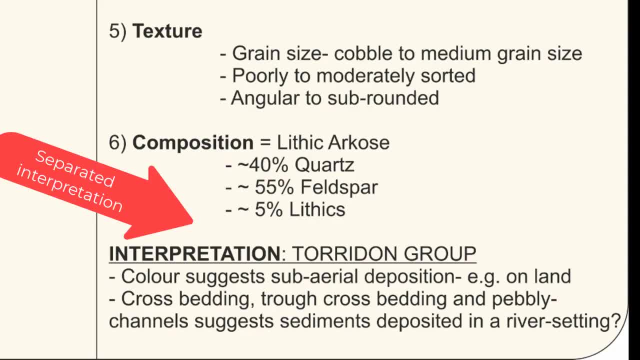 So finally I can now interpret what is my rock type here. I am pretty sure we are in the Torridon group, Especially from my previous observations at Clactol And along the shores of Loch Asin. The colour suggests we're in a sub-aerial depositional environment on land. 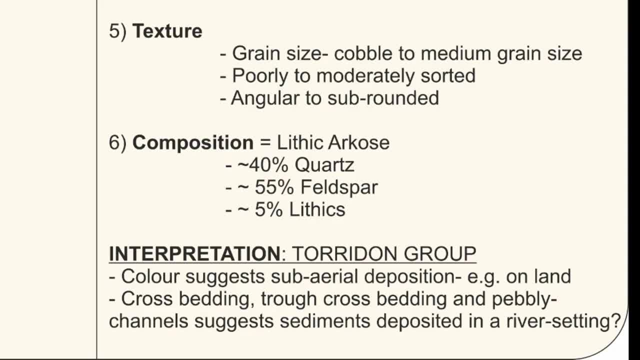 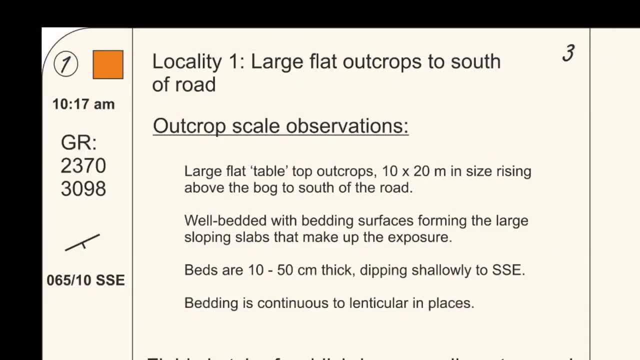 Cross bedding, trough cross bedding, pebbly channels suggest sediments deposited in a river setting. So I'm now happy that I have the Torridon. I can now colour this in on my map And also put a coloured square in the margin of my notebook. 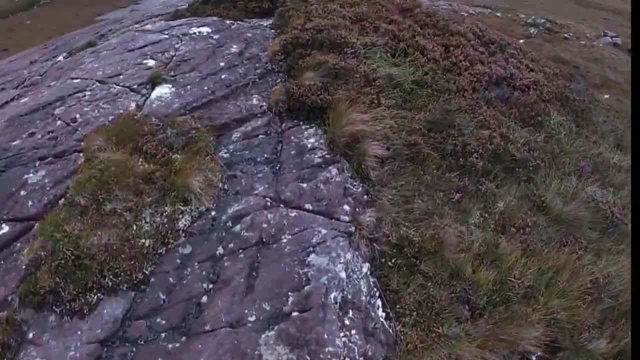 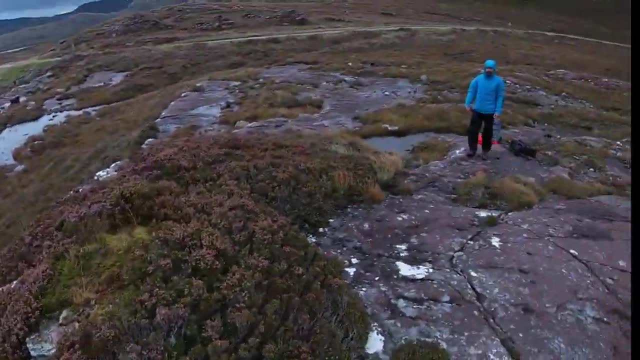 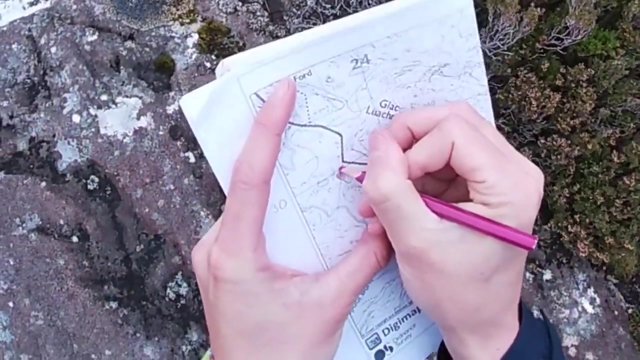 In order to fully represent this Torridon outcrop on my map, I am walking around trying to gauge the shape and size of the outcrop, Which I will then colour in on my map, Looking at how it forms in the landscape And how I'm going to represent that as a coloured outcrop on my map.